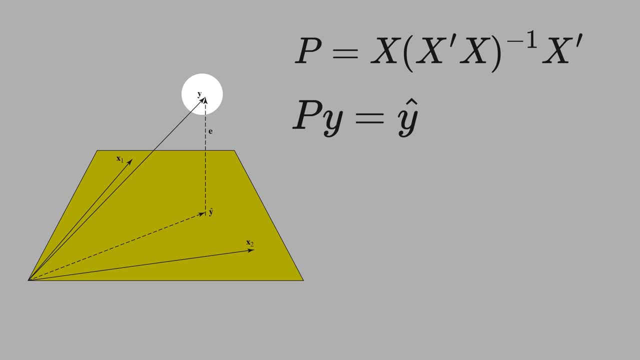 times y, you get the y hat. That means if I take this point, y, and multiply by P, I will get the y hat. here in the yellow plane. Let's show this mathematically. By definition, this is the matrix P. Then we multiply by y. And what is this term here? In the ordinary square, this is the. 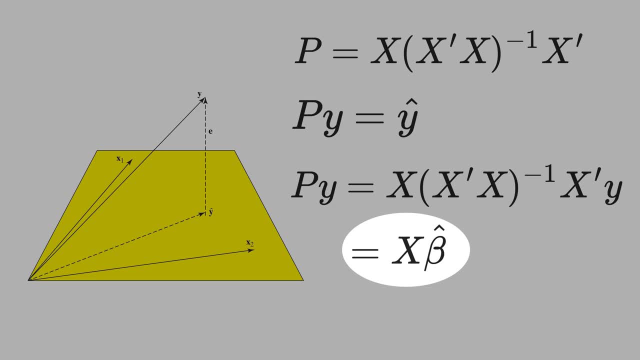 beta hat. And what is x beta hat? It is the definition of y hat. See that in ordinary square, y hat is the explanatory variables times the specific betas hat. Now let's show that Px equals x. This has to be intuitive because if x is already in the plane and you project on the plane, 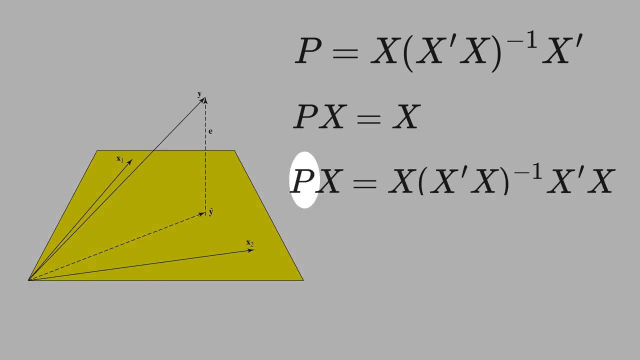 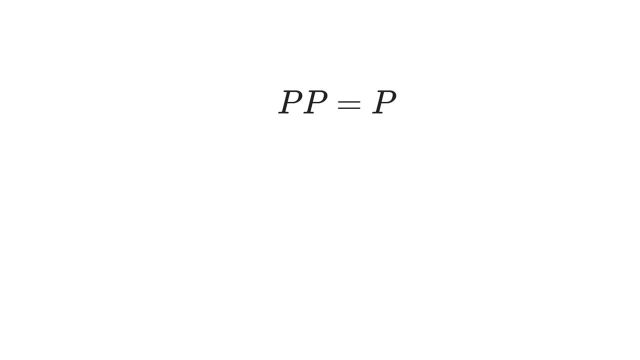 you are in the same place. Let's use the definition of P. Here is the definition of the matrix: P Then times x. We can cancel these two terms. Then you have Px equals x. Now let's prove that P is idempotent. That means P times P is equal P. Let's write the definition of: 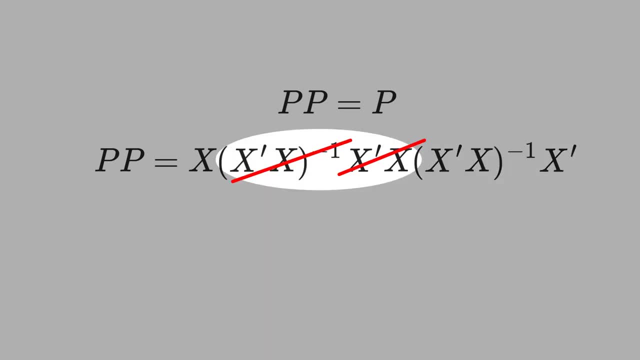 P And again the definition of P. here. Note that you can cancel these two terms here, And then you get the definition of the matrix P. What we are learning here will not only be useful for the ordinary square, But for other estimators as well, Like instrumental variables and the fixed. 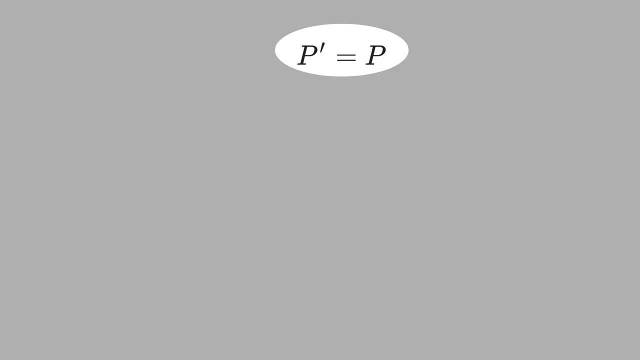 effect. Now let's derive that P is a symmetric matrix. That means P trace or P transpose, equal P Inside. here we have the definition of P and then we put the trace. Let's distribute the trace. See that you have to invert the x and then put the traces. This is the first trace. 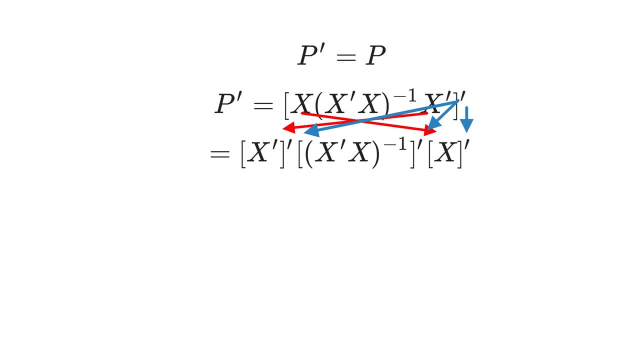 the second trace and the third trace. You might want to pause the video and analyze all these errors carefully. x trace, trace is equal x and the x trace is just x trace. See that you can switch the inverse and the trace. Now we have to invert the x to distribute the trace.